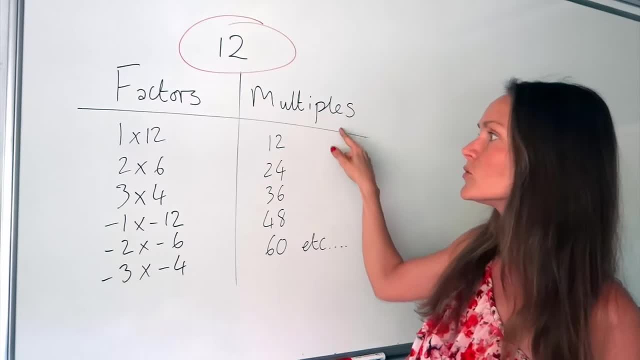 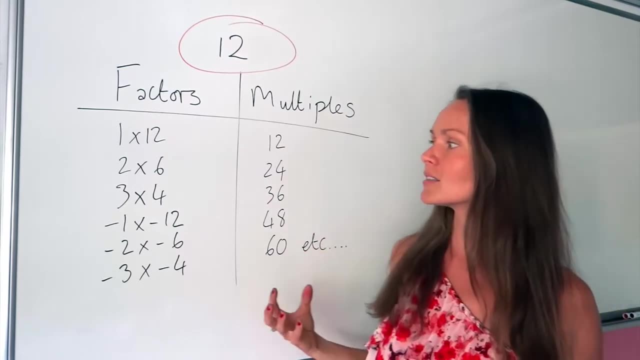 12 times table. So just remember, for multiples you have to multiply, OK. So all the numbers when you multiply 12, they're the multiples. So factors are going to be smaller but multiples are going to be bigger. 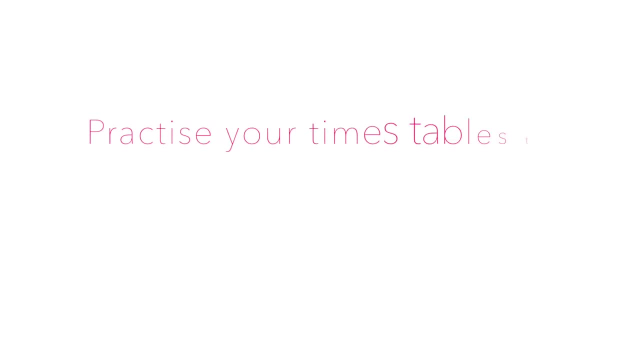 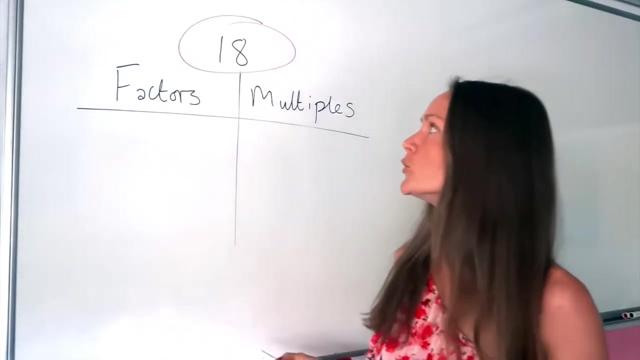 OK, I've got one more example to finish. OK, so here we go again. I've got a new number. This time it's the number 18.. And I'm going to start by listing the factors. So remember, these are the numbers that fit exactly into. 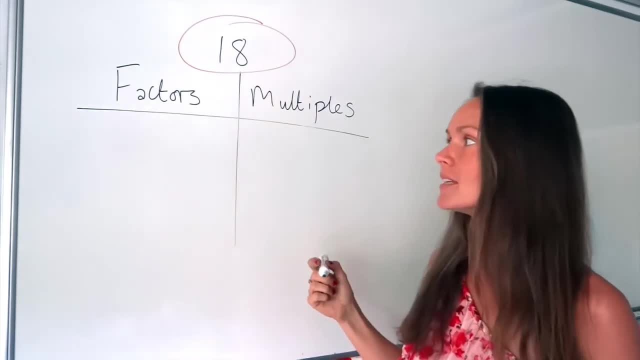 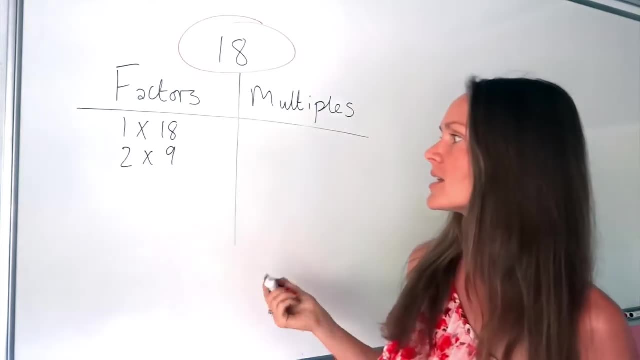 18.. So these are the numbers that we multiply to find 18.. So we've got 1 times 18,, which is 18.. So these are factors. We've got 2 times 9,, which is 18, and 3 times 6.. Well, the number. 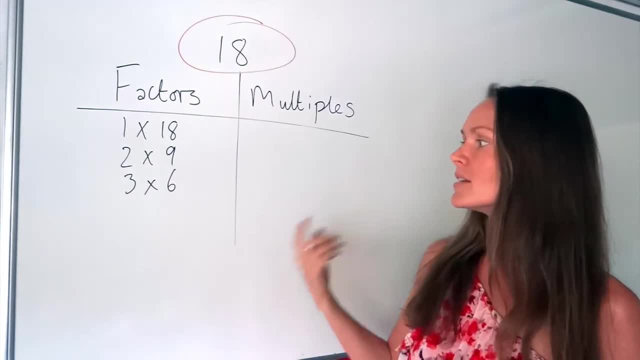 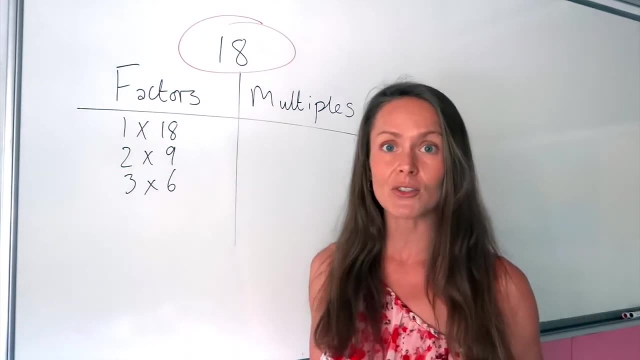 4 doesn't go into 18.. Neither does the number 5.. 6, we've already done So. I know I've included all of the factors there. So really you've just got to practice your times tables to get good at finding these factors. Don't forget you've also got the negative ones. We've also. 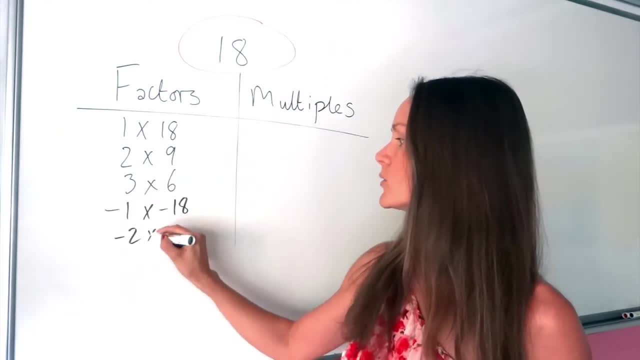 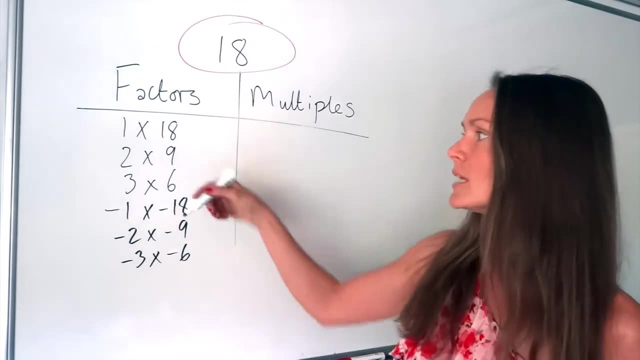 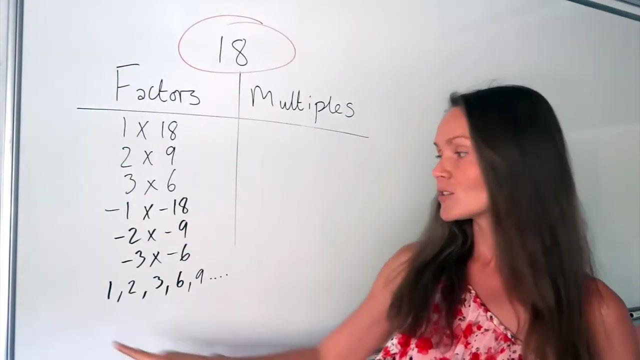 got negative 1 times negative 18, negative 2 times negative 9, and negative 3 times negative 6.. So if it asks you to list the factors, don't leave it like this. Just leave them written out like this, for example, And I'll just put dot, dot, dot. OK, So these are the 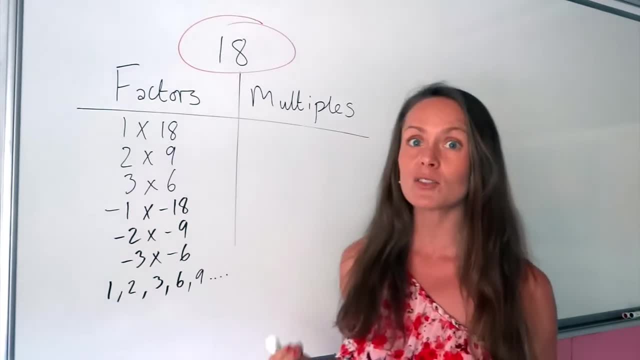 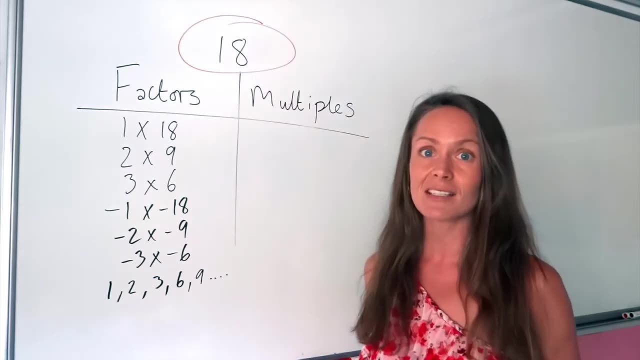 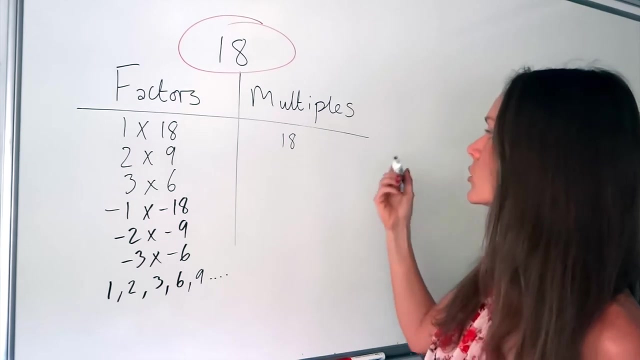 factors of 18.. Now for the multiples. So remember, to find the multiples you must multiply. So we're multiplying 18.. We're looking for the 18 times table To generate the multiples. So 1 times 18 is just 18.. 2 times 18 is 36.. 3 times 18 is: 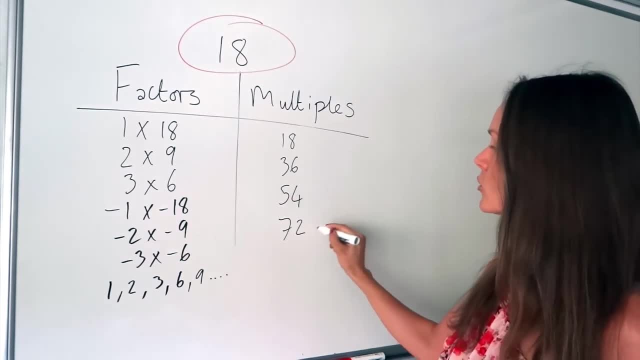 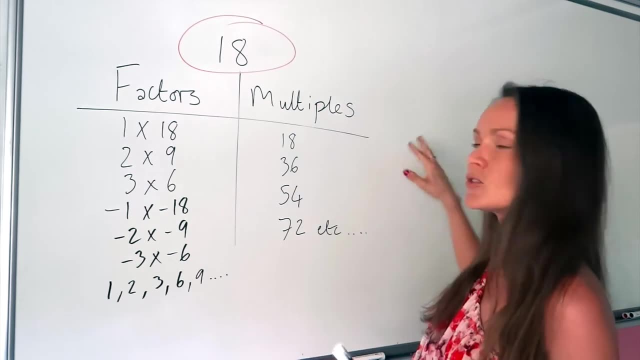 54.. 4 times 18 is 72, and so on. OK, I'm not expecting you to know your 18 times table. You might be able to use a calculator or just do your working out somewhere else, OK, So? 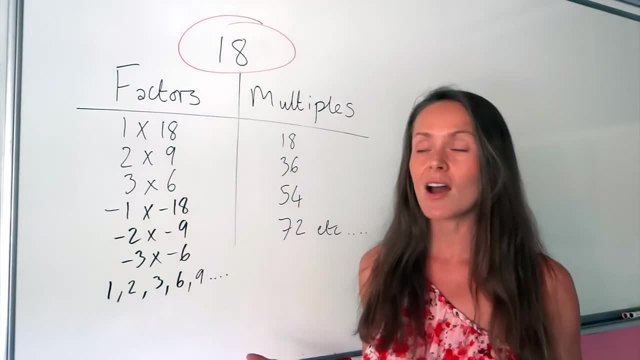 that's factors and multiples. And, like I said earlier, practice those times tables, Because if you're good at your times tables, you'll find these questions much easier.